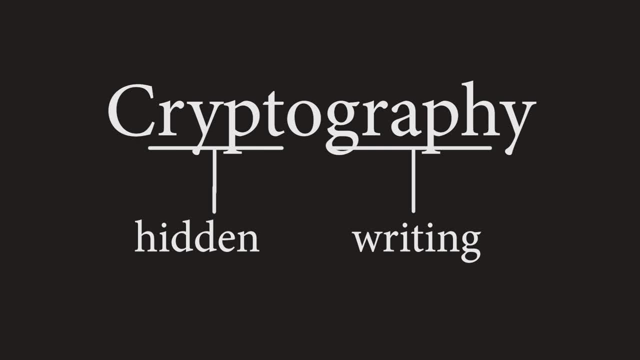 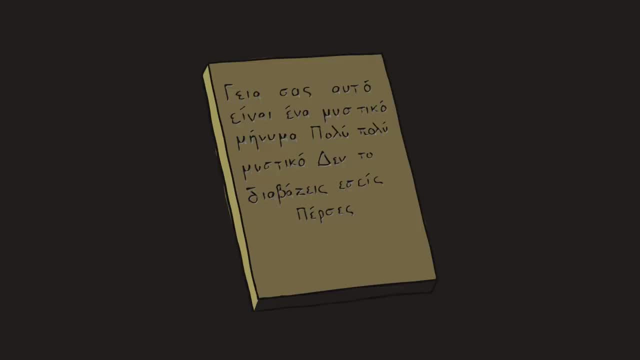 and some of the earliest forms of secret writing come from ancient Greece as well. Herodotus, the father of history, as he is known, described a way of hiding writing by putting a message on a wooden board and then covering it with a layer of wax. During Greece's war with Persia in the 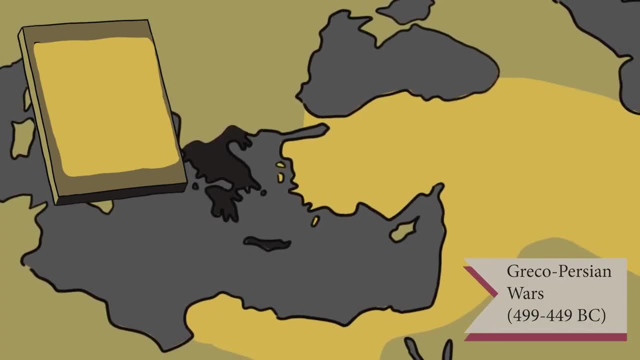 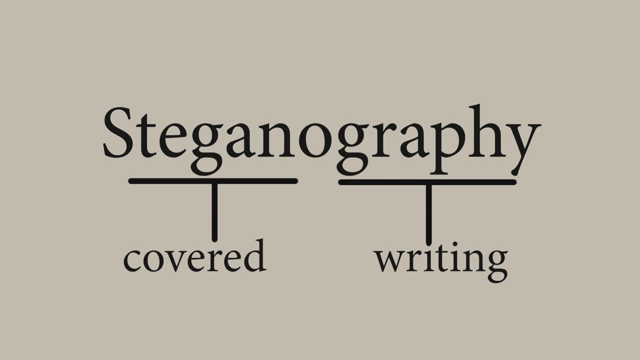 5th century BC, this approach was used to send military correspondence. This sort of concealment is known as steganography, meaning covered writing. It was common all over the ancient world, from Greece to China, But, as you can probably guess, this approach has some issues. 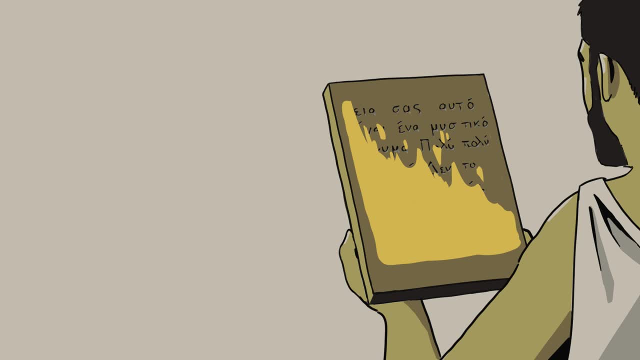 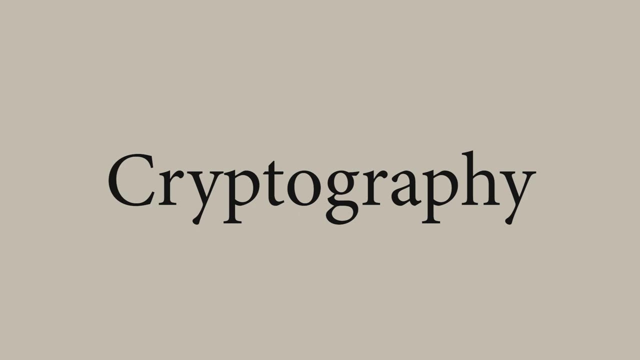 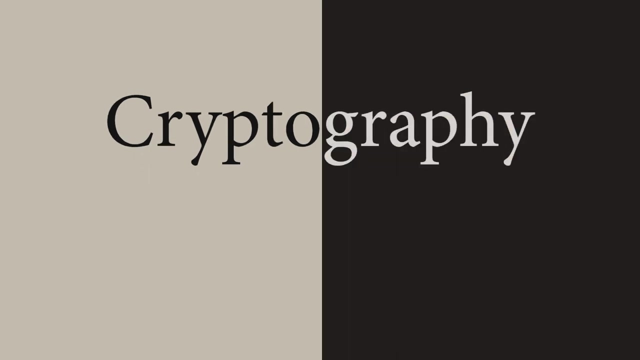 The main one being that, if the message is discovered, its contents will be easily revealed. This dilemma gave rise to cryptography, which doesn't hide the existence of a message, but instead hides its meaning. Cryptography can be broken down into two subtypes: transposition and substitution. 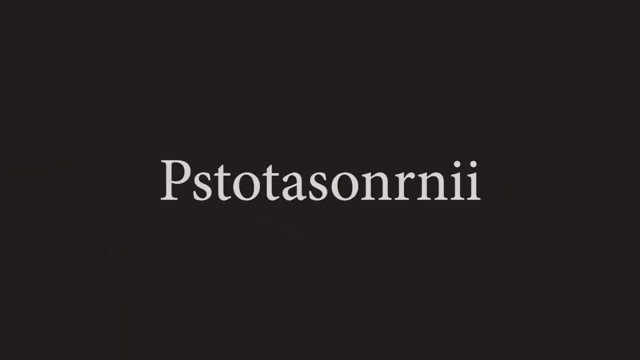 Transposition is when a document is rearranged, creating an anagram, And if a document is rearranged, creating an anagram. Transposition is when a document is rearranged, creating an anagram. Transposition is when a document is rearranged, creating an anagram. 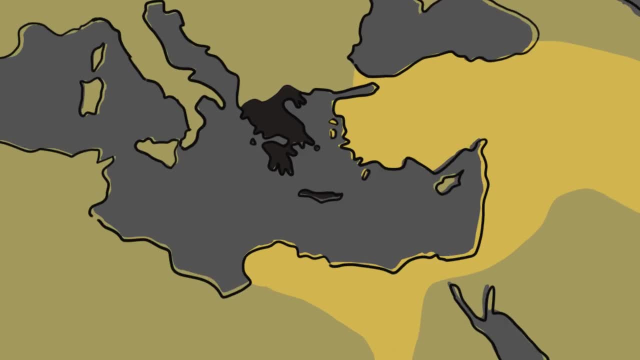 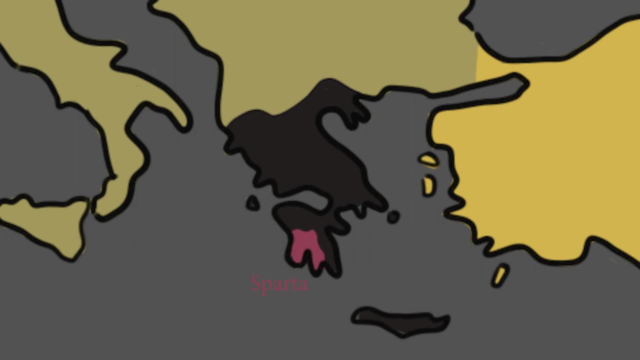 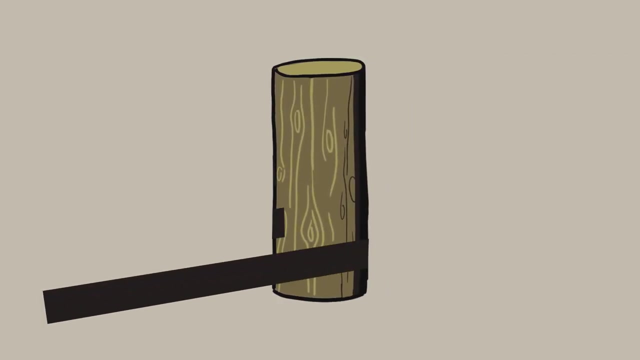 It is the earlier form of cryptography. An early historical example is once again from ancient Greece, specifically the city-state of Sparta. The Spartans used a device called a skytale to hide their military communications. It consisted of a strip of leather wrapped around a wooden rod. 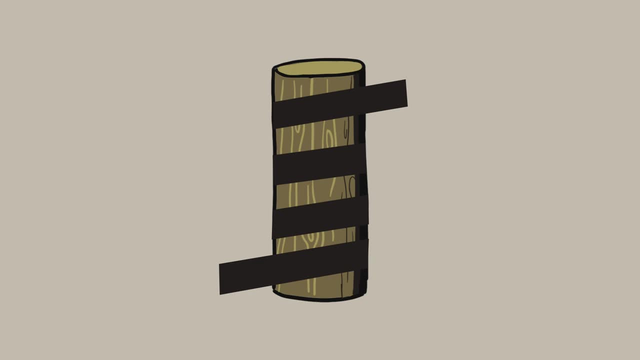 The sender would write his message on the leather as it was twirled around the rod like so, When unfurled, the message would seem like a jumble of letters, But once the receiver wrapped the strip around an identical rod of their own, the message would become clear. 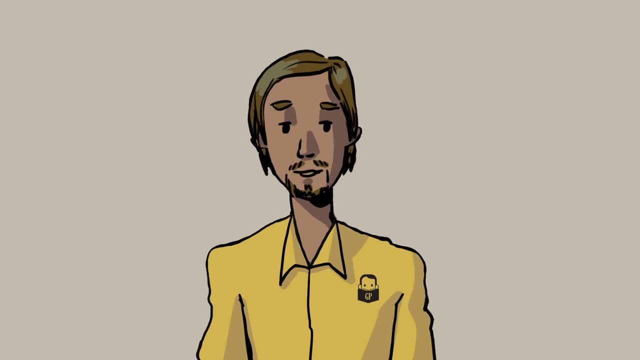 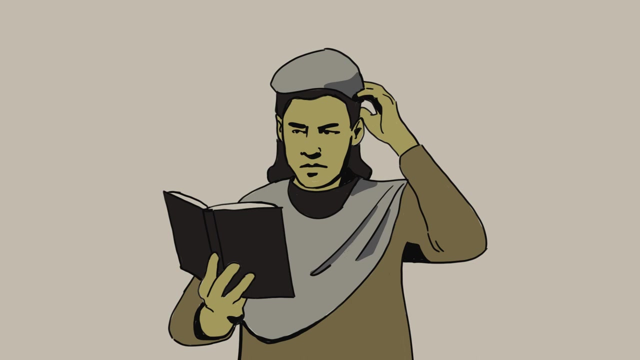 Transposition has some major flaws, though. For one, a short message has a limited number of scramblings. For instance, the word dog can only be rearranged five ways And larger messages while more difficult to disentangle for an interceptor. 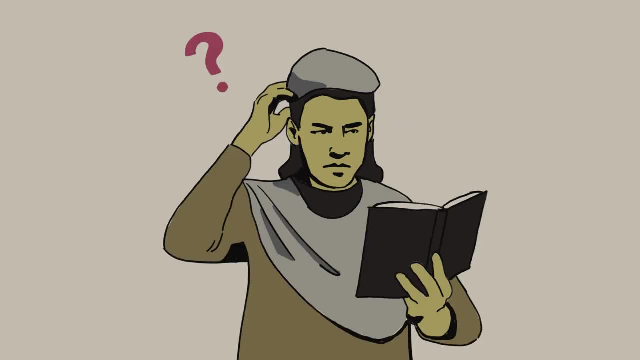 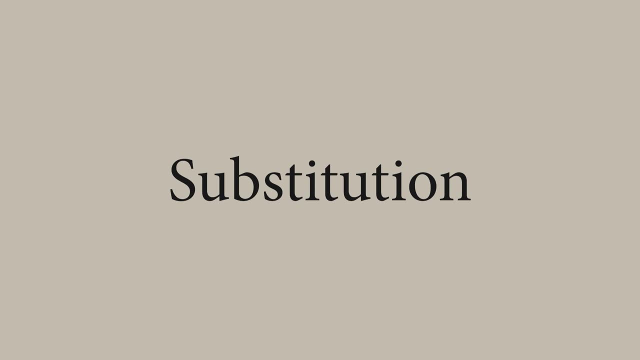 will also be too difficult for the intended receiver as well. Because of this, cryptography was created by substitution. Substitution rather than rearranging the letters in a message, instead replaces the letters altogether. The most famous substitution cipher is the Caesar cipher. 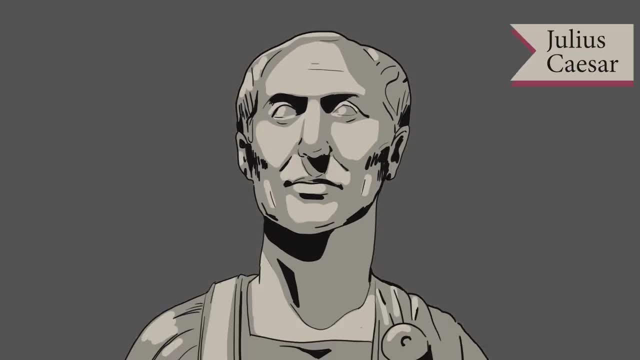 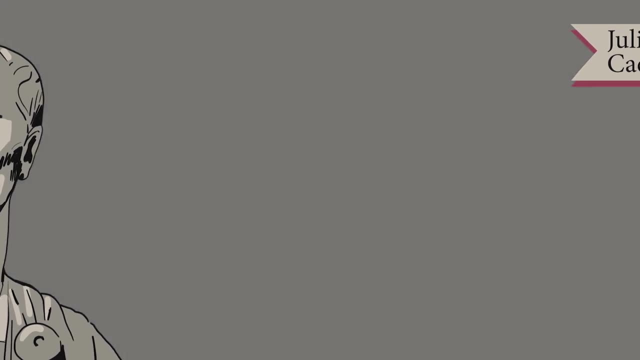 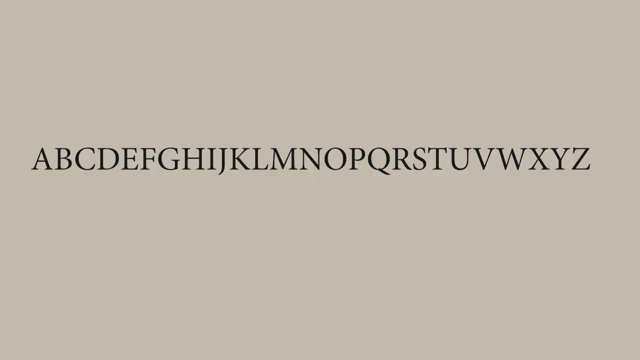 As the name implies, it was used by the Roman dictator, Julius Caesar during the Gallic Wars in the first century AD. The Caesar cipher, also known as the Caesar shift cipher, replaces any given letter with the letter in the word letter three spaces down the alphabet. This is why it's called a shift cipher, because the cipher 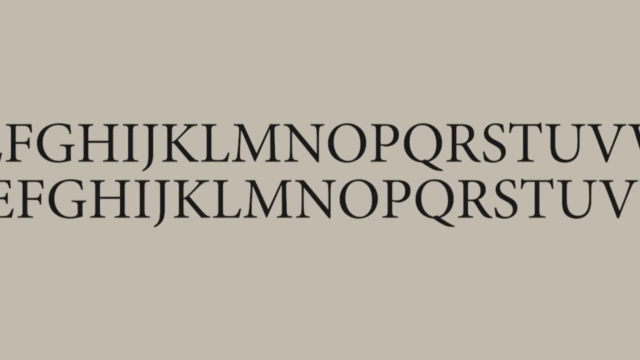 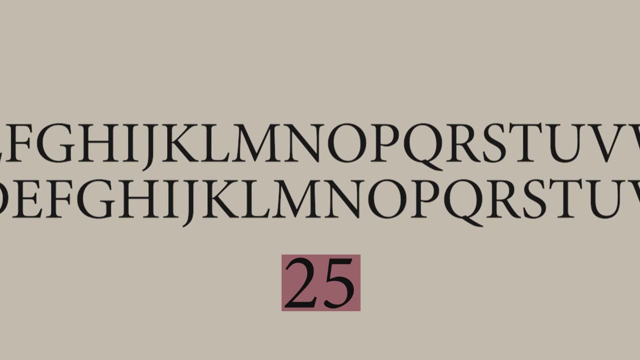 alphabet is simply the plain alphabet, shifted three spaces like. so. Traditionally, Caesar favored a shift of three, but, as you can see, you can shift the alphabet as many times as you want. Accordingly, there are 25 variations of the Caesar cipher. This is pretty good, but if someone knew, 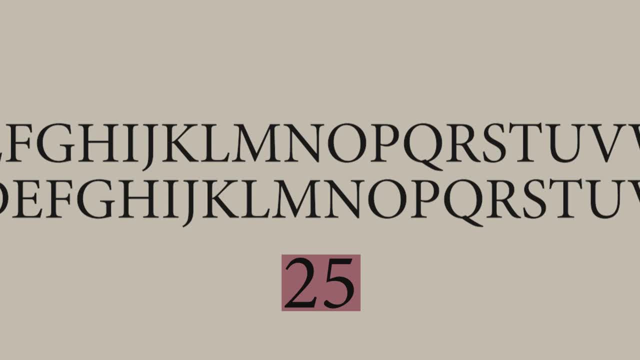 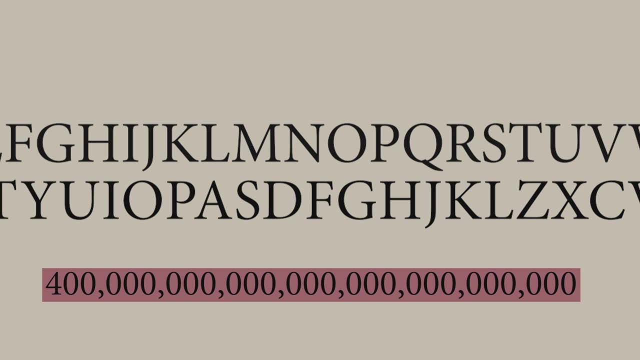 you were using a Caesar cipher to encrypt your message. they could brute force their way through by checking all 25 shifts, But if you scramble the alphabet at random instead of simply shifting it over, you get 400 septillion, that's 400 followed by 24 zeros different permutations. So obviously a. 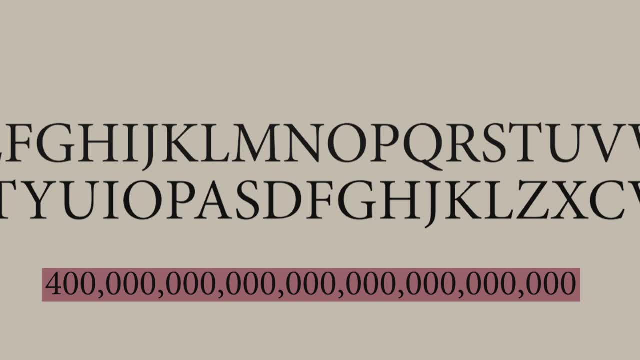 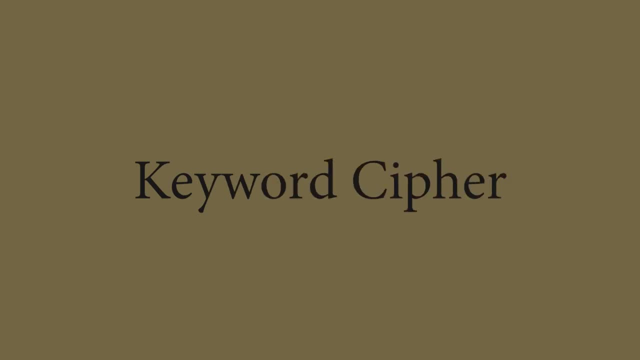 wannabe code breaker would have no chance brute forcing his way through such an encryption. However, a totally random shift would be a good idea. A random arrangement of the alphabet would also be difficult for the receiver of a message to remember. One solution to this problem is a keyword cipher, Essentially the sender and receiver of a secret. 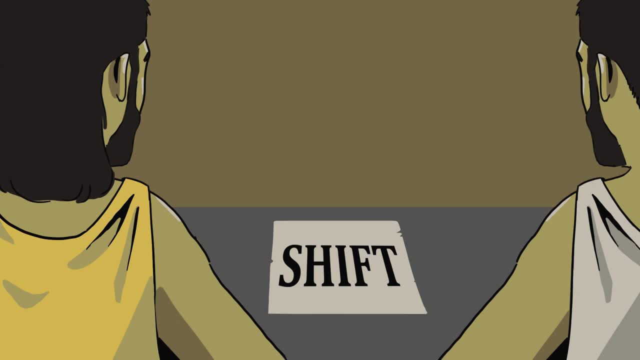 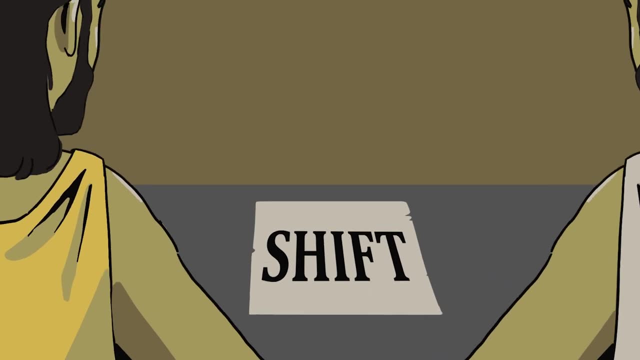 message would agree on a keyword and that would be used to construct the cipher alphabet. Let's say our keyword is shift, Easy enough to remember, right. So the cipher alphabet would be made by spelling shift, then filling in the alphabet according to the last letter of the word. 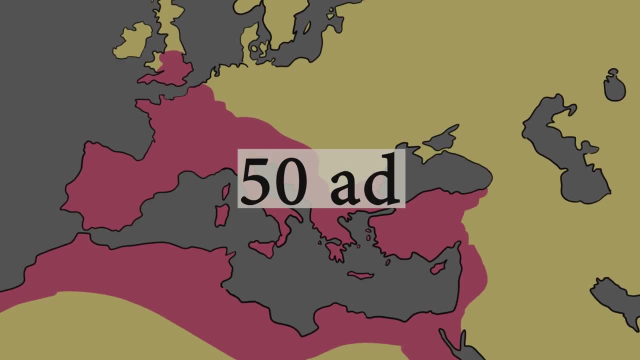 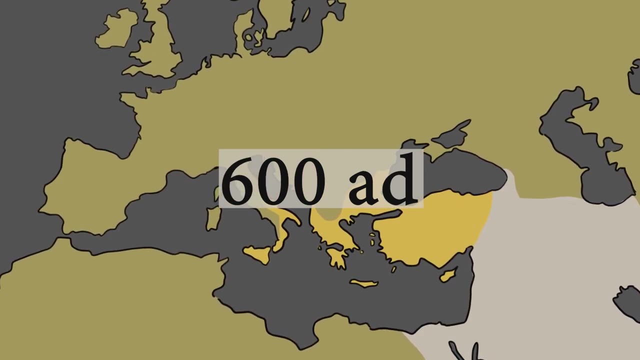 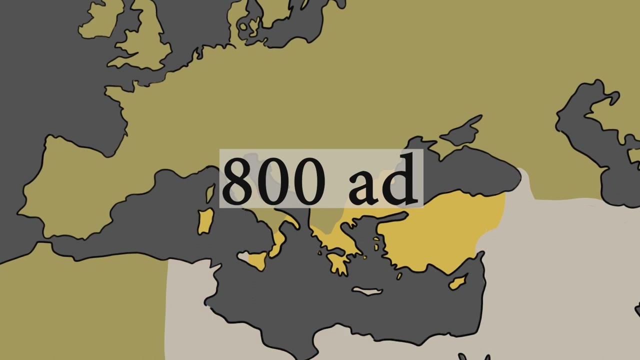 In this case T like this. Throughout the rest of the Roman Empire's history and into the 6th century AD, these simple ciphers, broadly called mono-alphabetic substitution ciphers, were used to great success, That is, until the 8th century. 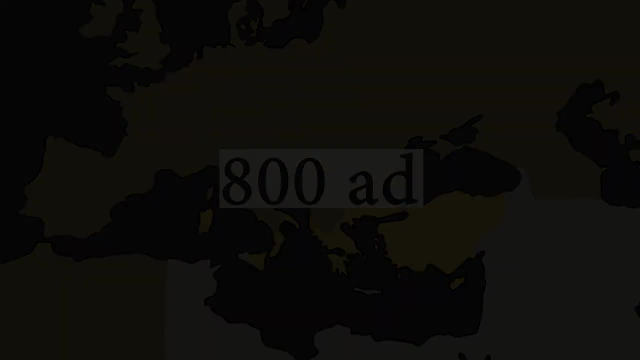 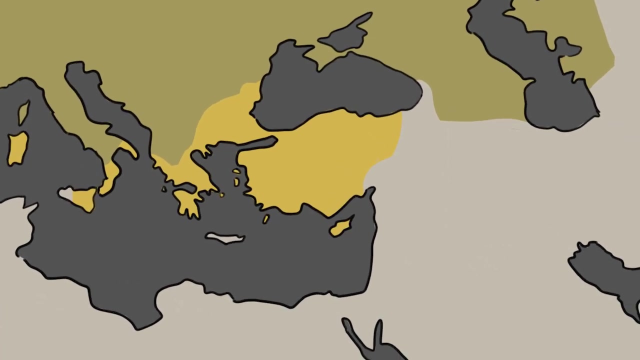 when a group of ingenious scholars found a way to break through these puzzles. In the Middle East, about a hundred years after the death of the prophet Muhammad, a new dynasty took power called the Abbasid Caliphate. This new leadership heralded what 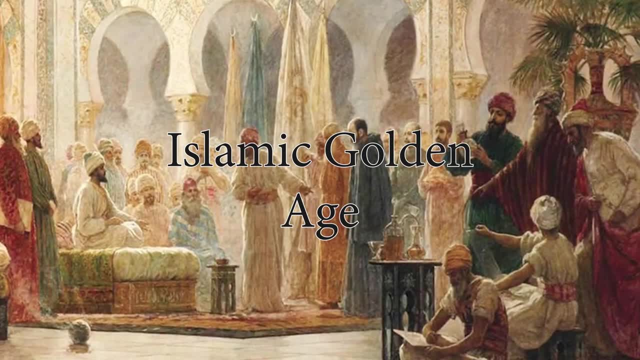 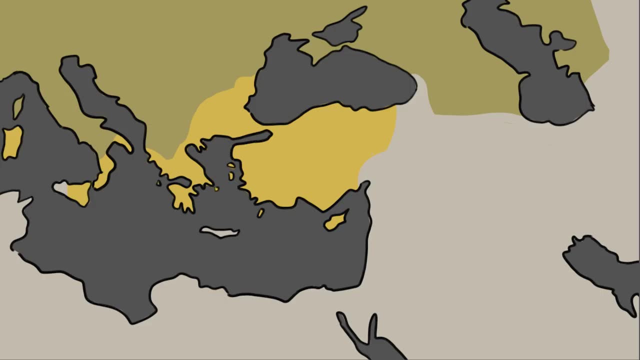 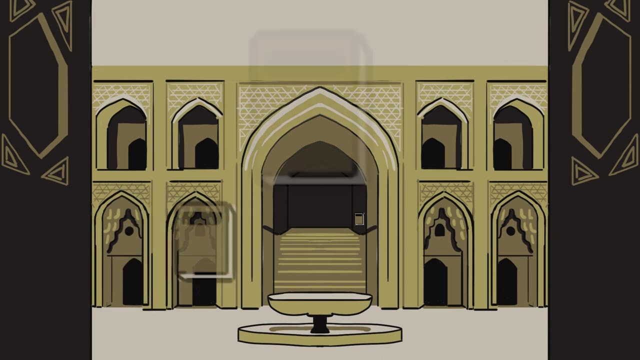 is called the Islamic Golden Age. This time of prosperity and peace was the perfect cradle for an intellectual age. Islamic scholars centered in the Baghdad House of Wisdom collected works on astronomy, medicine, alchemy, music, mathematics and more. They also added their own knowledge. 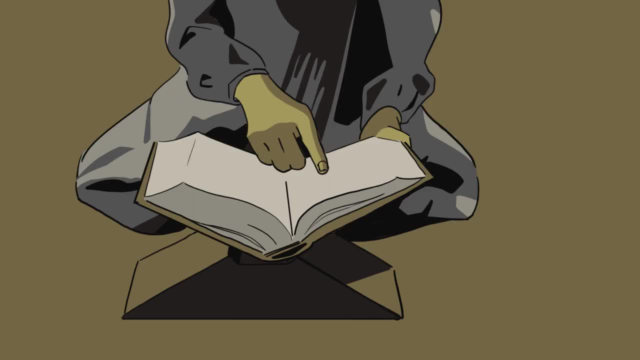 to the collections. They also added their own knowledge to the collections During this time. During this time, Muslim theologians were studying the Quran and the hadiths. They wanted to know which revelations came earlier in the Quran and which hadiths were. 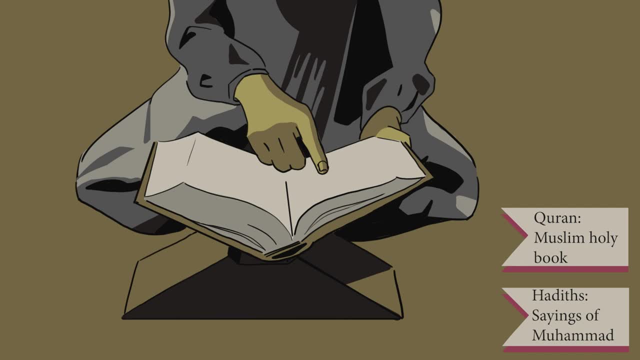 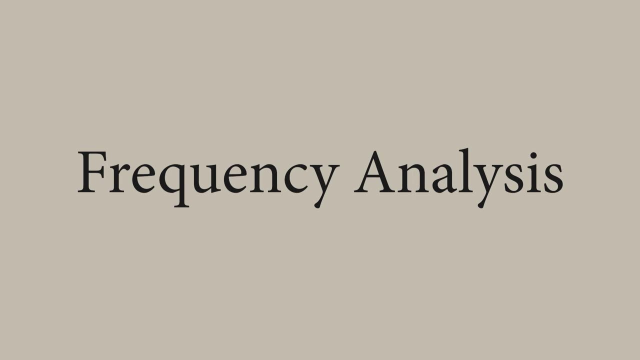 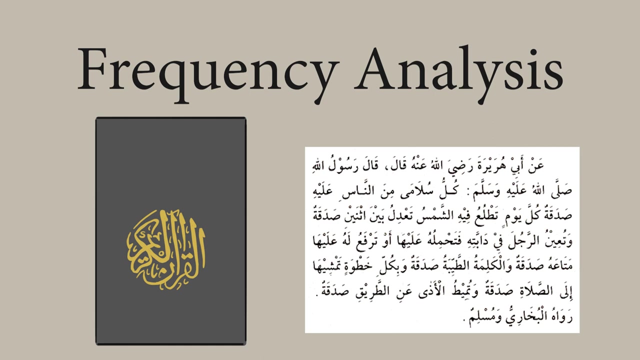 genuine and which were not. They did this by using new statistical and linguistic techniques. Chief among them was called frequency analysis. Scholars saw how often words were used in the Quran and the hadiths, and this investigation would show whether the linguistic styles and etymological idiosyncrasies of the documents 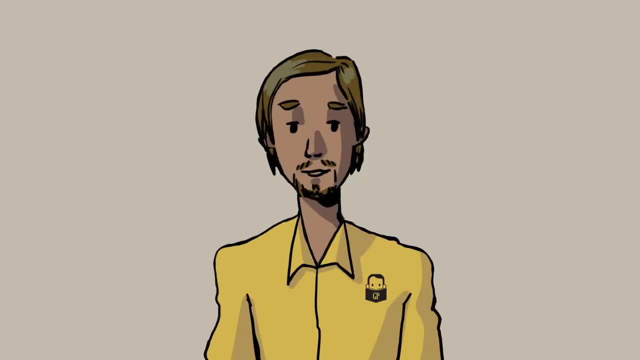 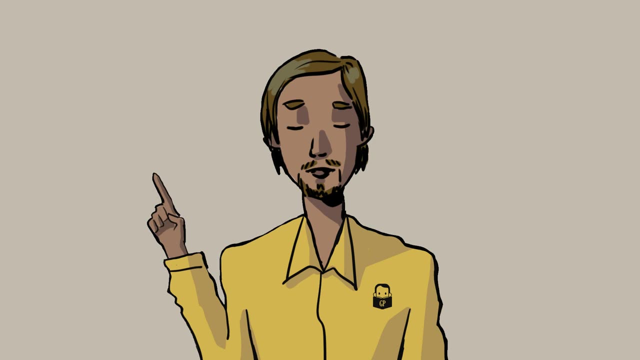 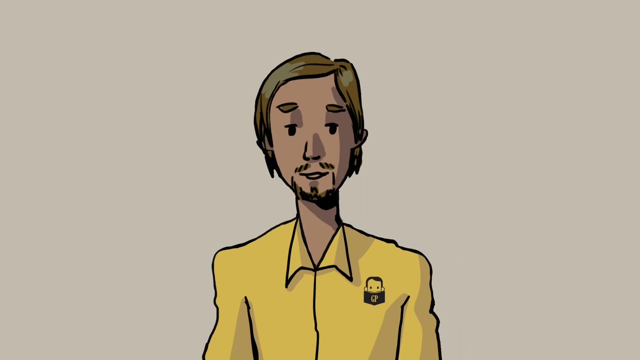 were in line with Muhammad's. They also used this analysis on individual letters, not just words, and in doing so discovered that certain letters were more frequently seen than others. The first scholar to realize this frequency analysis could be used to break ciphers was 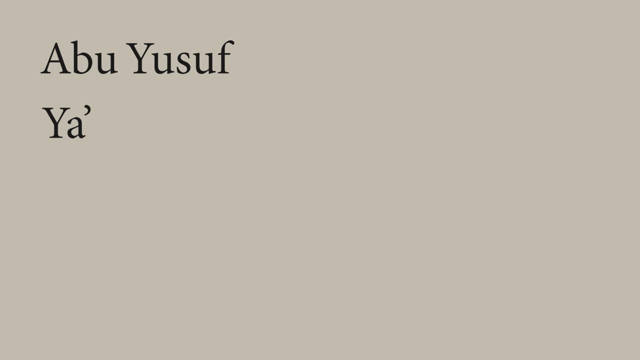 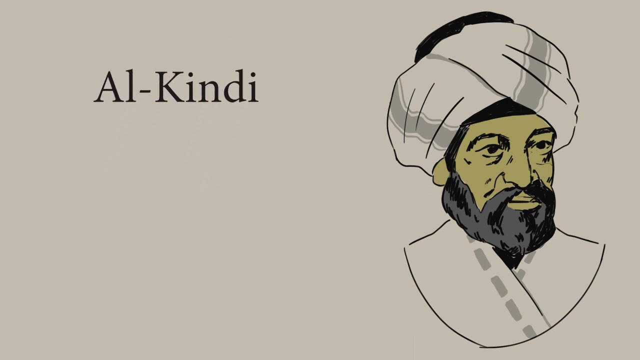 a man named Abu Yusuf Ya Yaqub Ibn al-Mu'min. Uh, this guy, We'll just call him al-Kindi. He was a very important philosopher who wrote hundreds of works on all sorts of subjects, from mathematics to music to medicine. 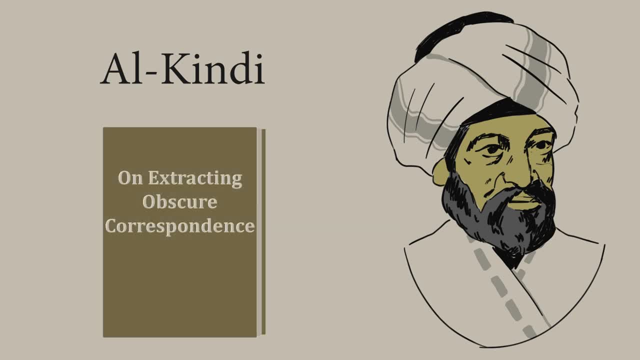 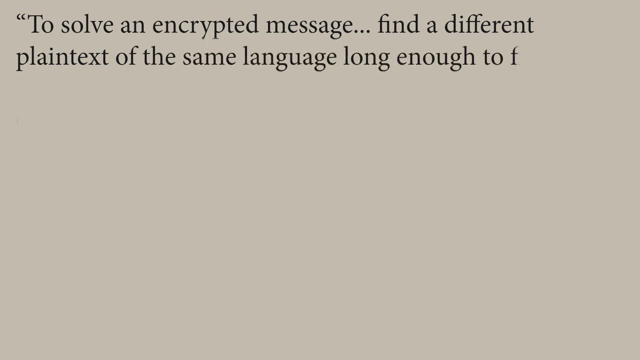 He also wrote a treatise on cryptanalysis, the study of code-breaking. Here's a quote from his book which concisely explains his ingenious technique To solve an encrypted message: find a different plain text of the word of the same language long enough to fill one sheet or so, and then count the occurrences of each. 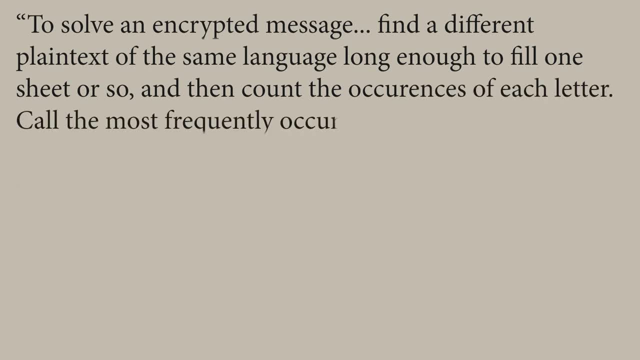 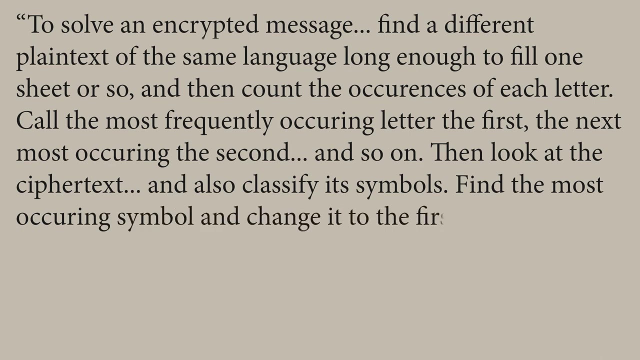 letter. Call the most frequently occurring letter, the first, the next most occurring, the second, and so on. Then look at the ciphertext and also classify its symbols. Find the most occurring symbol and change it to the first letter. The next most common symbol is changed to the form of the. 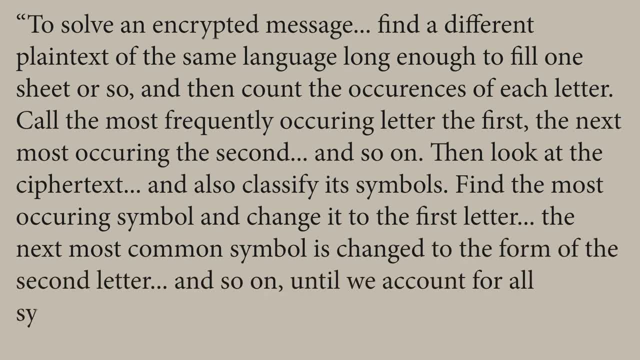 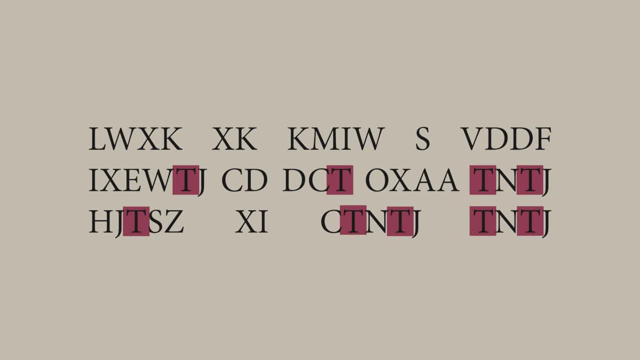 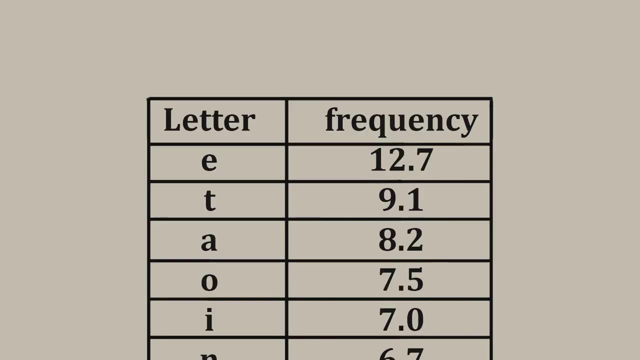 second letter and so on until we account for all the symbols of the cryptogram we want to solve. Essentially, find the most occurring letter in a cipher and assume it is the most occurring letter in the normal alphabet. In English, the most common letter is E, followed by T. 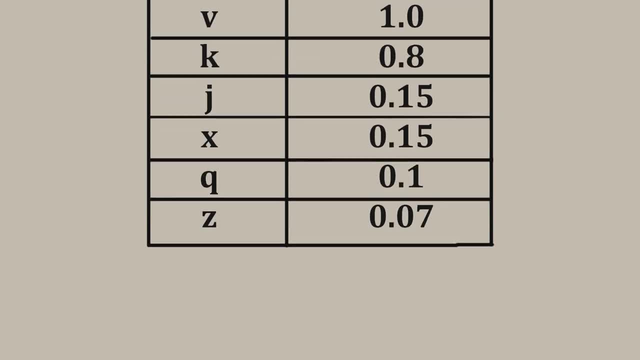 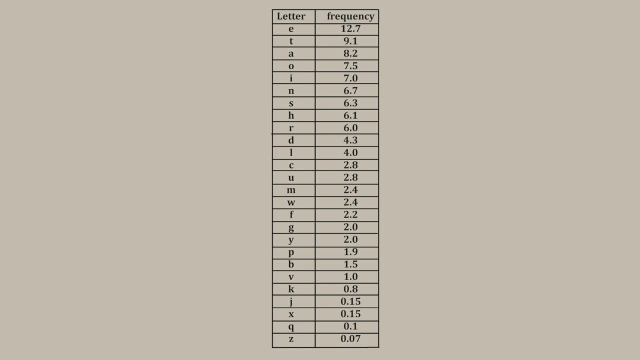 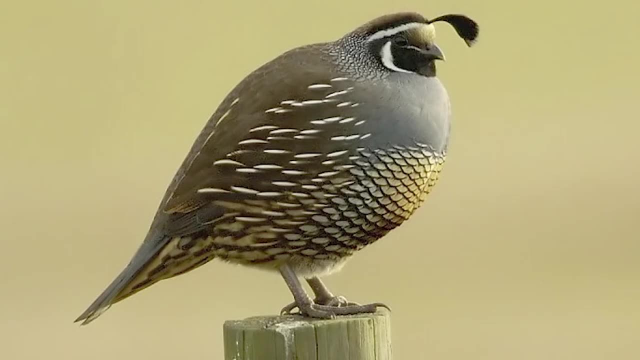 and so on, while the least common are Q and Z. Here's a handy chart. As you might be able to guess, this method can't be used unconditionally. Say you're deciphering a C- secret treatise on zebras, xylophones and quails. You wouldn't expect to see these letters. very frequently, and that would probably throw a wrench in your analysis. Still, an intelligent cryptanalyst can break pretty much any mono-alphabetic substitution cipher using frequency analysis, even when letters don't line up perfectly with their statistical likelihood. Heading back west. 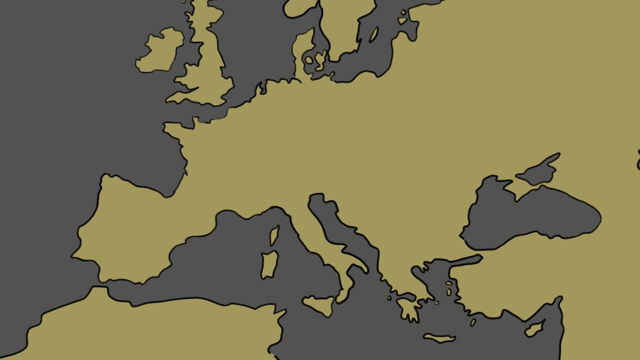 Europe had been going through the dark ages. While the dark ages is generally a term I dislike when it comes to cryptography, it is fitting, as medieval Europe had little interest in the subject. That was until the Renaissance, With the outpouring of interest and study in the 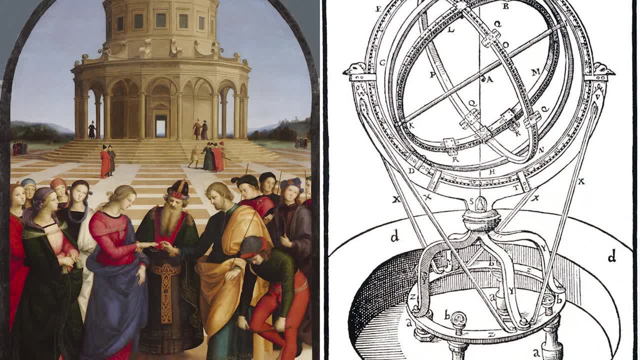 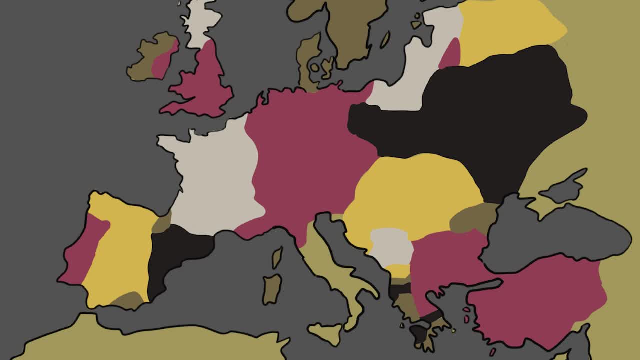 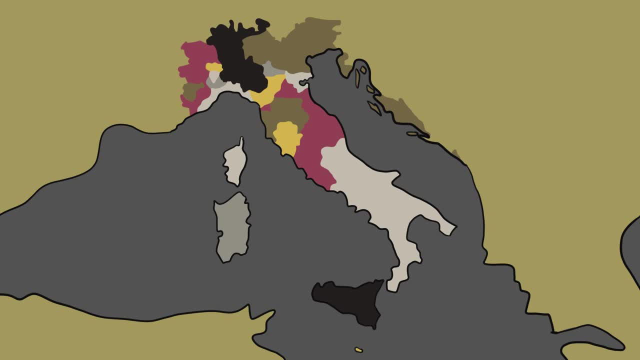 arts and sciences. during this time, the study of cryptography was reinvigorated too. The political situation in Europe was also responsible for the renewed interest in keeping communication secret. This was especially true in Italy, which at the time was not a unified country. 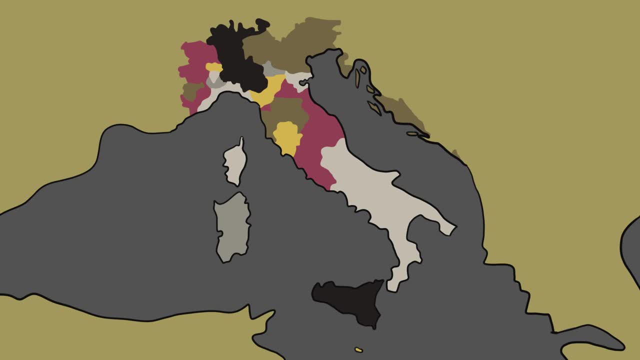 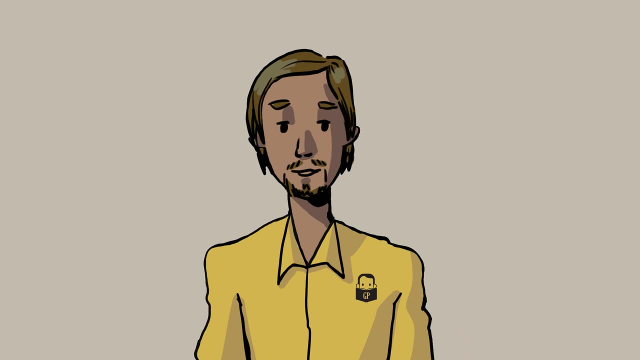 but a mishmash of small kingdoms and city-states, all constantly bickering with each other. So because of this political intrigue, mixed with the leaps forward in scholarship, cryptography became a burgeoning industry. By the 15th century, almost every court in 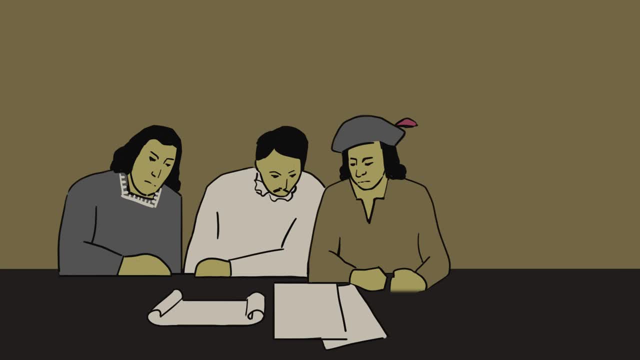 Europe had a cipher office and every ambassador a cipher secretary. But with the Islamophobia of the 19th century, the cryptography of the 19th century became a major issue. The cryptography of the 19th century was a major issue, But with the Islamophobia of the 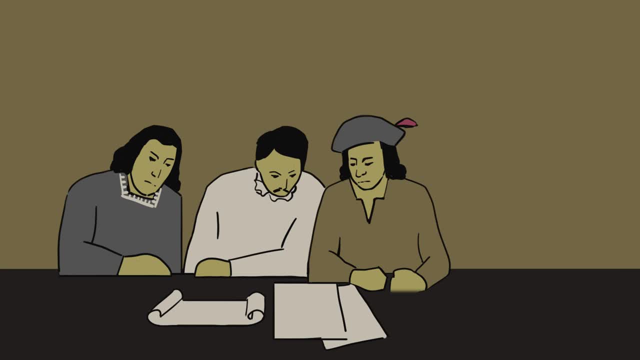 19th century, the cryptography of the 19th century was a major issue. But with the Islamophobia of the 19th century, the cryptography of the 19th century was a major issue. The Islamic code-breaking techniques having been brought to the West, the cryptographers were still at a disadvantage. 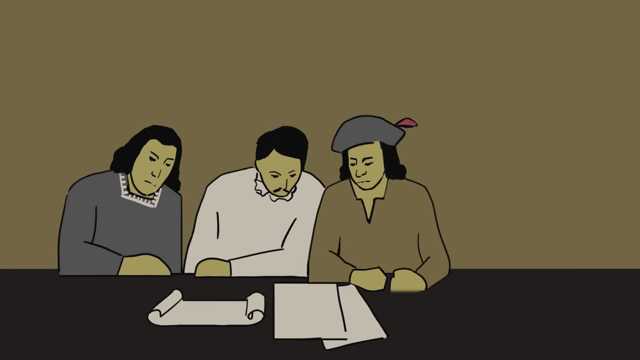 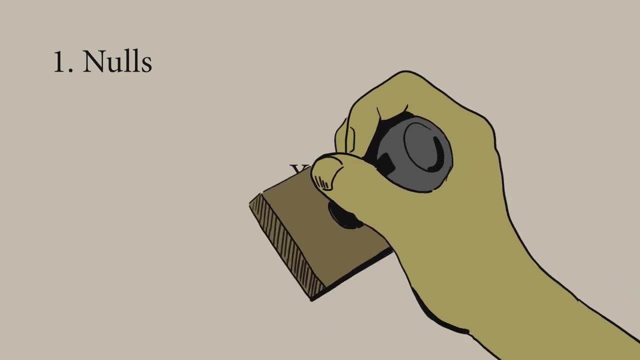 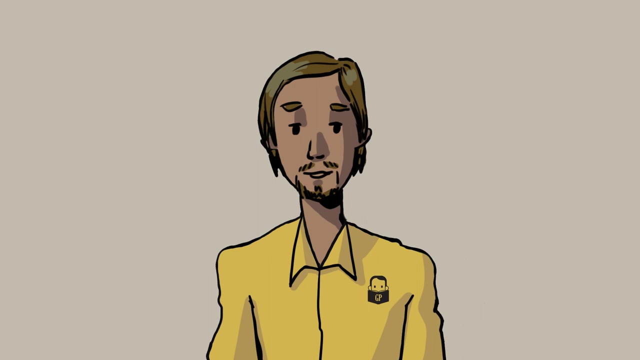 They needed new innovations to trip up the cryptanalysts. The first was the introduction of nulls. Nulls are symbols put into a cipher that have no meaning. Let's say you had a cipher made from numbers 1 to 50.. A quick side note: you may think that a cipher made from symbols or 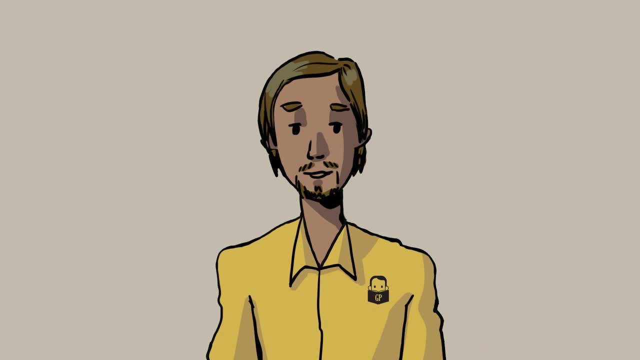 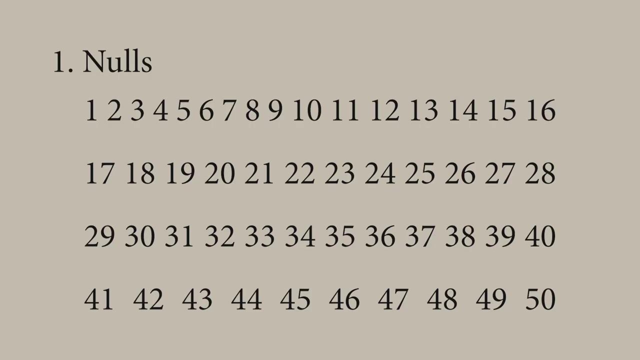 numbers instead of letters would be more difficult to solve, But they're not. Frequency analysis works just fine, regardless of what images are used. Ciphers using things other than letters existed for centuries before this. I just hadn't mentioned them. So a cipher made from 1 to 50.. Well, seeing as there are only 26 letters in the English, 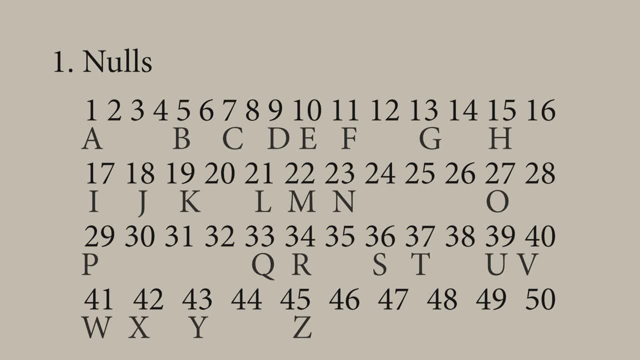 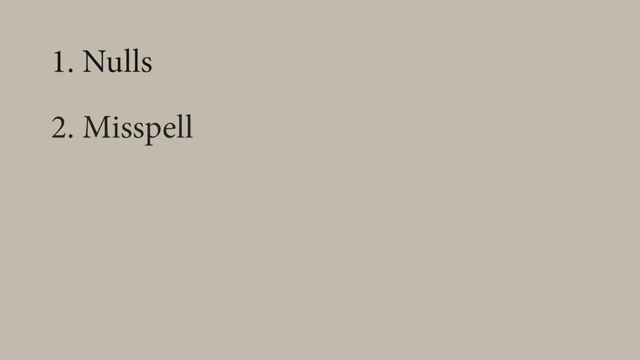 alphabet. only about half of these numbers would actually correspond to letters. The rest would be nulls. The second innovation was to simply misspell the encrypted message, so that when a cryptanalyst uses a cipher, he or she will not be able to read the encrypted message. The second: 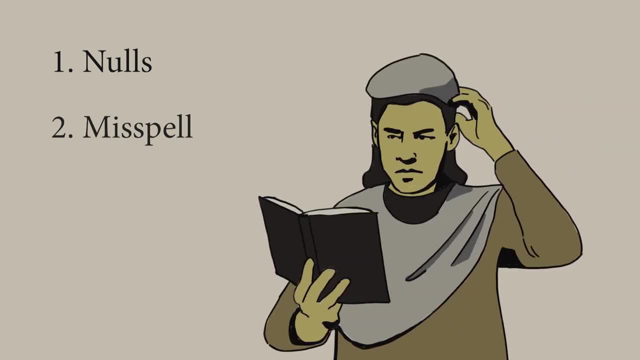 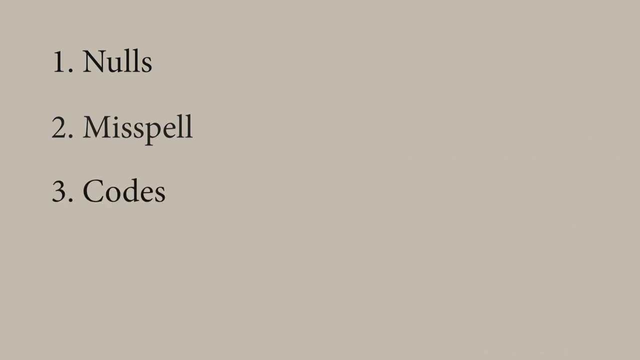 innovation was to try to break the cipher. he would slowly uncover misspelled words and then stop thinking he's going about it all wrong. And lastly, the introduction of codes In cryptography. codes and ciphers are two different things. Codes are words that mean other words, like a codename. Codes replace words. 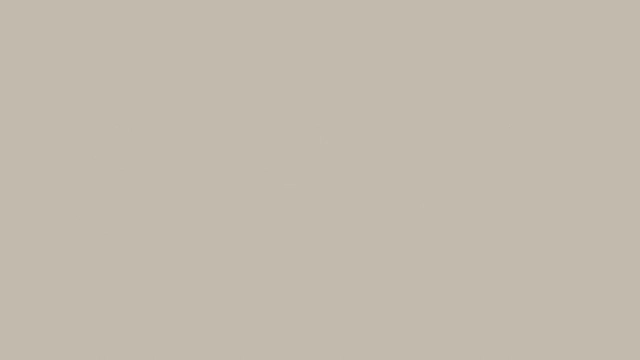 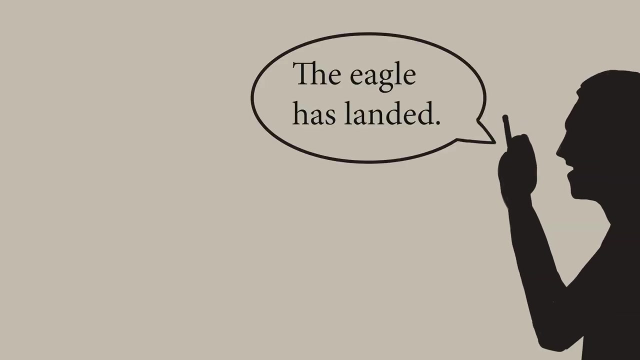 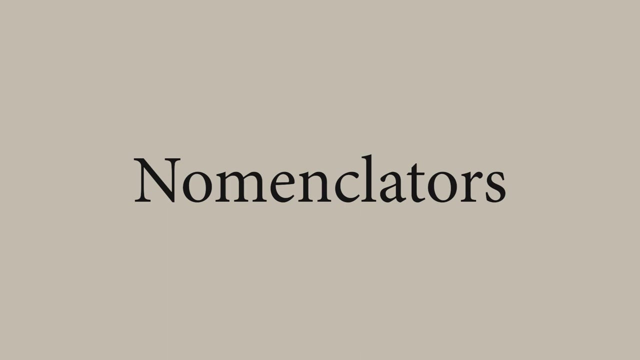 while ciphers replace letters. Codes are obviously most useful when applied to a short message, But not so good with long messages. Because of this limitation, cryptographers started using nomenclators. Nomenclators are a mix between ciphers and codes. Essentially, 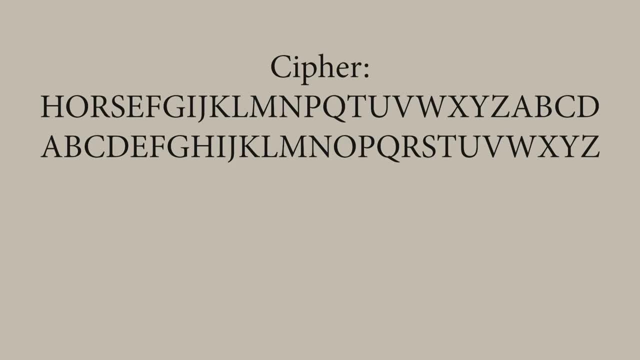 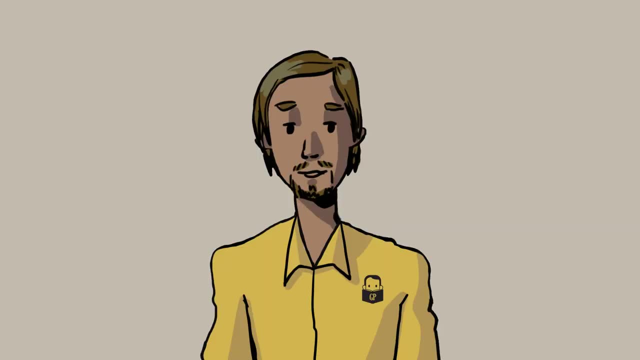 a message would be encrypted using a cipher while also using a small list of important code words. As impressive as all these new techniques were, a cunning and intelligent codebreaker could figure out the nulls, ignore the misspellings and understand the code words through context. 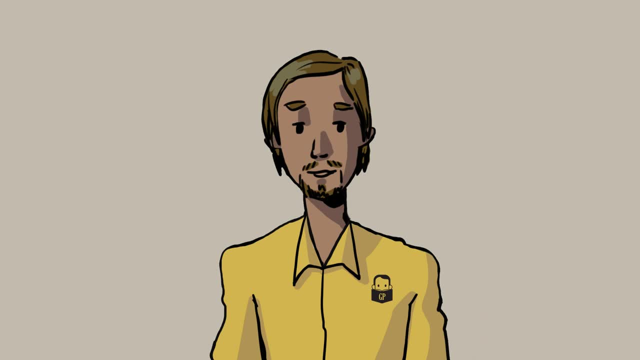 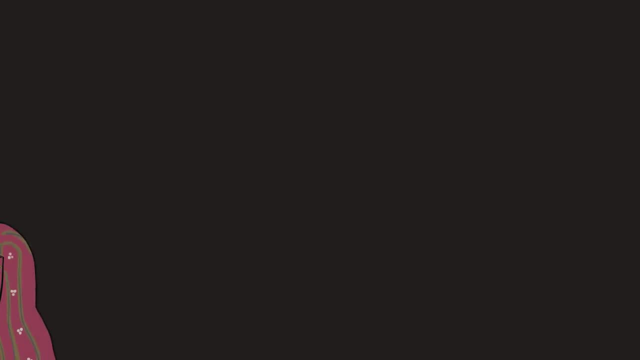 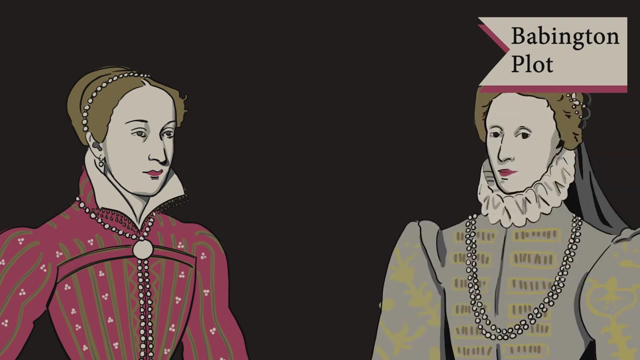 For decades, cryptanalysts still had the upper hand, as shown in the case of Mary, Queen of Scots. While imprisoned on trumped up charges, Queen Mary took part in the Babington Plot, a plan by English Catholics to kill Queen Elizabeth and replace her with Mary. She had corresponded with the conspirators using a cipher. 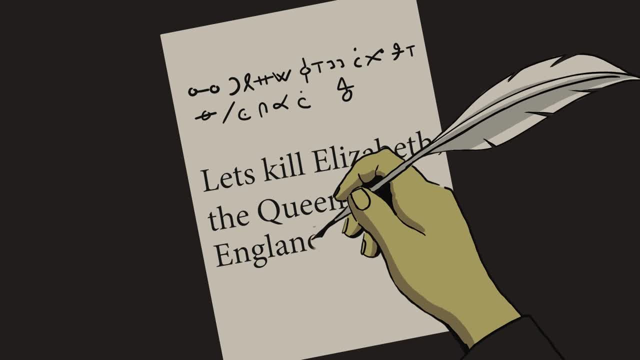 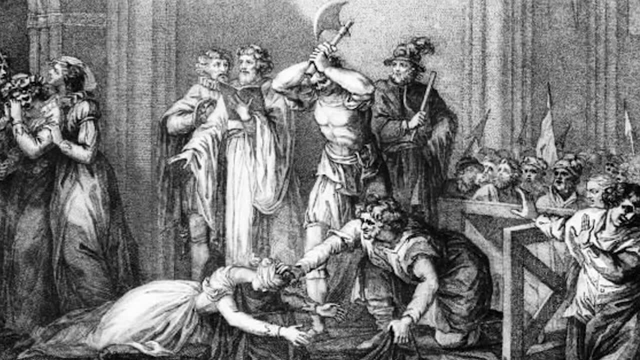 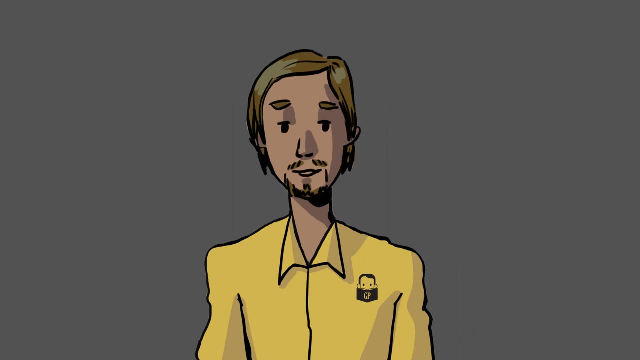 which was unfortunately broken by English cryptanalysts, proving Queen Mary guilty. She was executed on February 8th 1587.. So clearly, cryptographers needed a better system And in the 16th century, a Frenchman named Vigenere would come up with it.